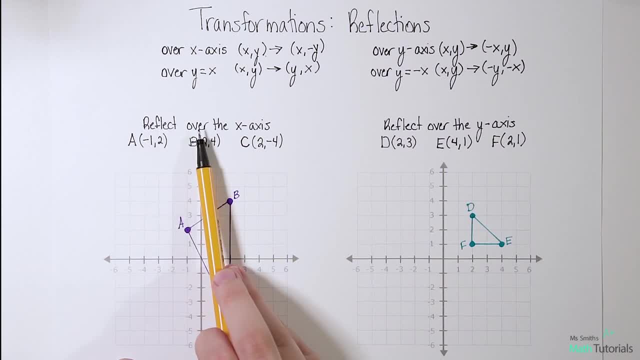 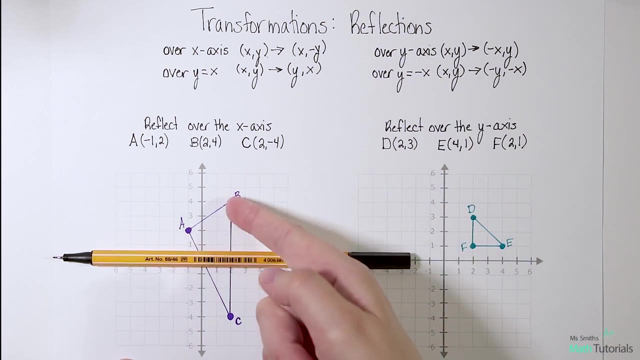 So let's start. let's try the first one: Reflection over the x-axis. It wants us to take this shape, this triangle abc, and reflect it over the x-axis. Now, the x-axis is right here where my pen is, So that means b will be reflected. 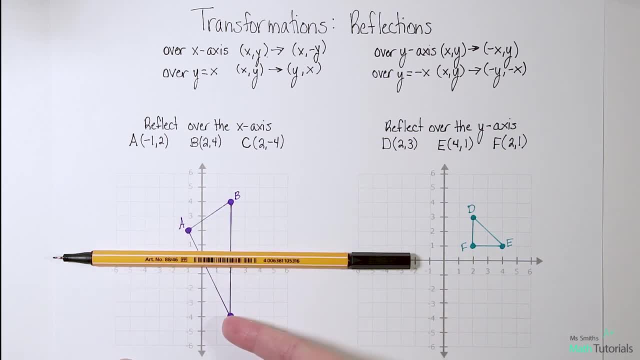 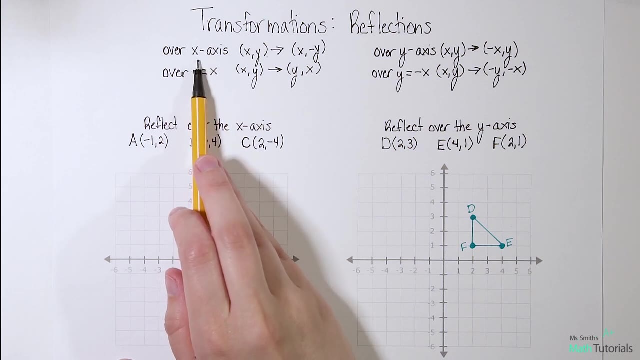 down here. a will be reflected down here, c will be reflected up here. So it's kind of interesting the way this is going to flip on itself For a. currently it sits at negative one two. Well, following that rule for a reflection over the x-axis, I need to leave the x where it is. 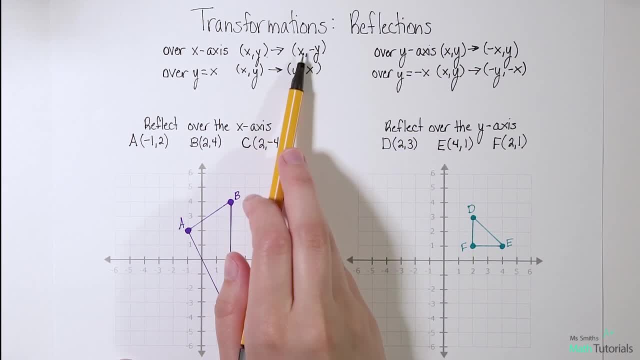 with the sign it has and the y: I'm going to flip the sign. That's what it means. when it says negative y, It means flip it, Okay. so if it's positive, it's going to become negative. If it's negative, it's going to become positive. You do whatever the opposite is. So for this point a, 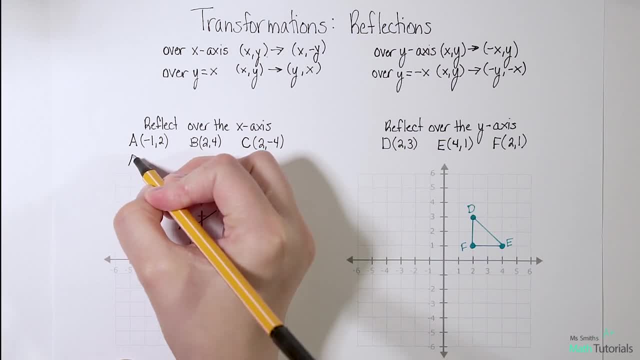 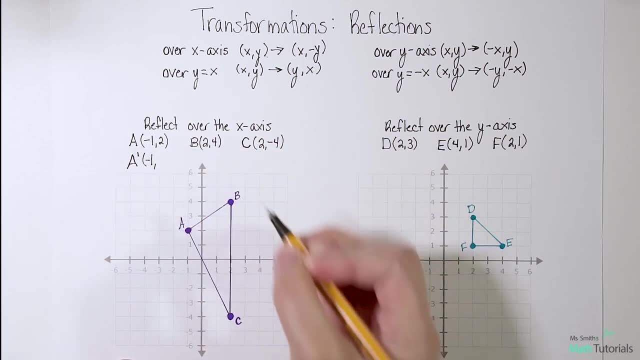 negative. one, two x is going to stay the same. Now we're going to do the same thing. We're going to create an, a prime, A new a x will stay the same and the y is going to flip sign. So this two will. 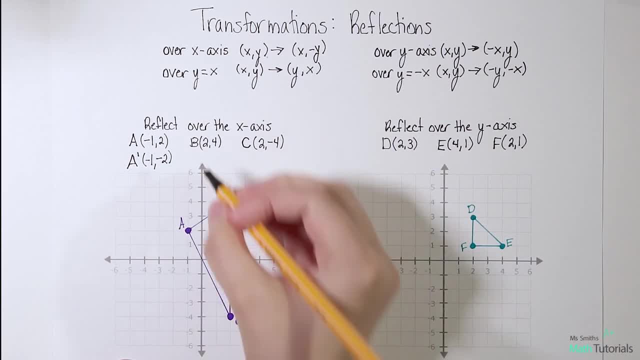 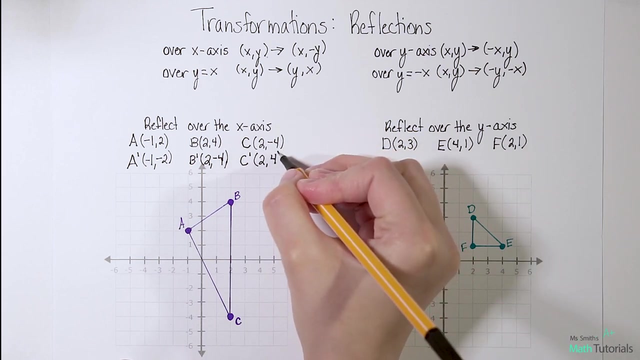 become a negative. two Now for b prime: same rule: x will stay the same, y will flip sign. All right. now for c prime: x will stay the same, y will flip sign. So notice, it was negative, Now it's positive Changes. So now I've got my new. 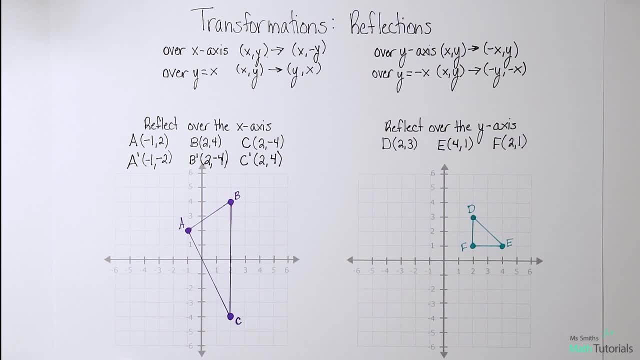 reflection image that I need to plot and and look at and verify that that is a reflection. So a prime falls at negative one, negative two. Oops, I don't mean to do that line. All right, so this is our a prime. Our b prime falls at two negative four, which is the same place as this c. So I'm just going to kind of. 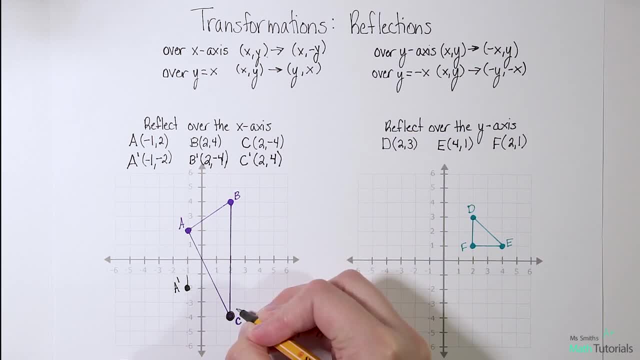 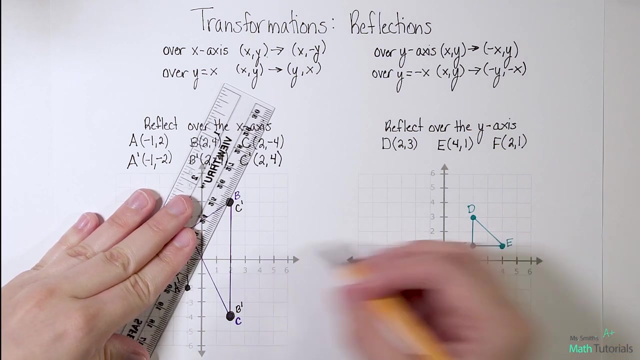 darken around it and we'll call that b prime And then the c prime falls at two positive four. So, again overlaid with the b, I'll just darken it and that is c prime, All right, so let me connect the dots. Let's see that. 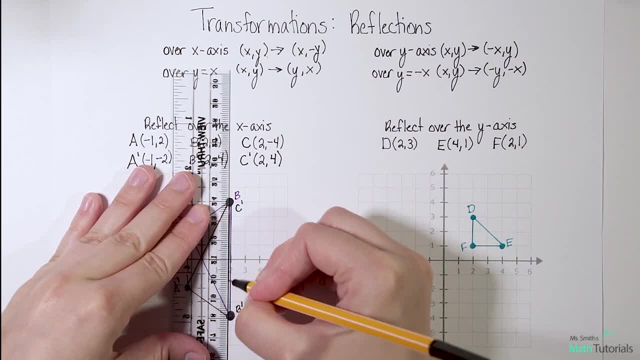 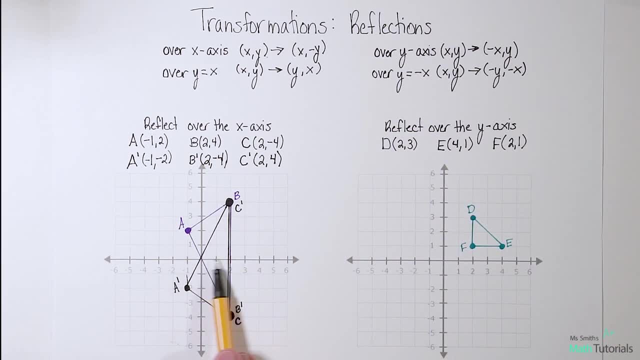 So you see how this image is reflected. It's almost like the y. the x axis is a mirror and we have a mirrored image around the x-axis. let's look at this one. this one asks us to reflect this turquoise triangle over the y-axis. it does. 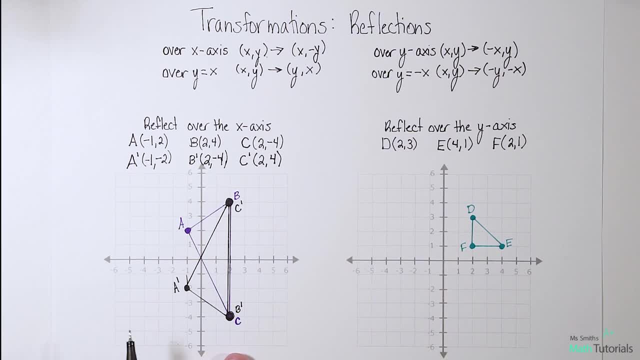 already give us the points of where that triangle currently is and we just need to take each point and reflect it over the y-axis using this rule. so the rule is: x- y becomes negative x- y. so that means this time the x is going to flip the sign, the y will stay the same. so for d, 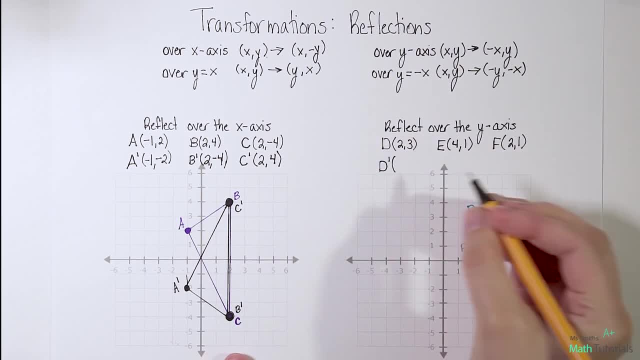 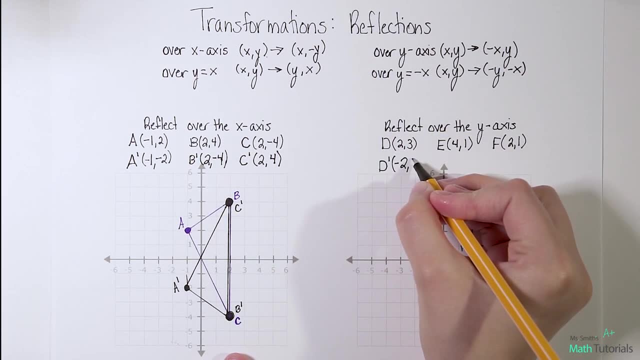 we're going to create a d prime. the x is currently positive two, so we're going to make it negative two and the y is three, so we're going to leave it three. for e prime, the four is currently positive, so he's going to become negative. 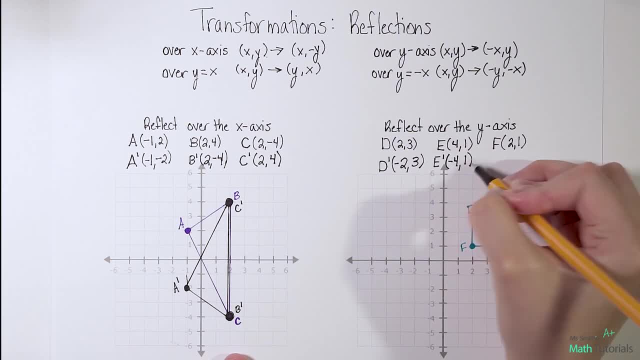 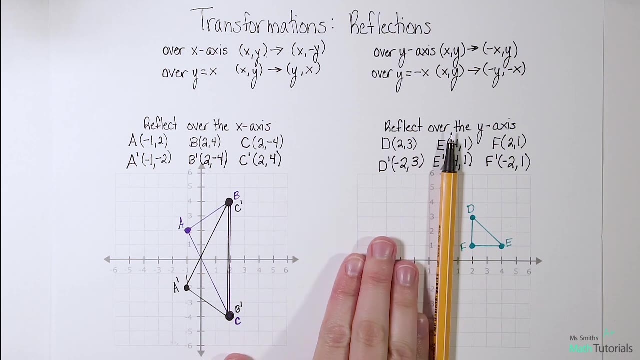 so he's going to become negative. the y is positive 1, so he stays positive. 1 for f prime. the two will become negative and the one will stay the same. this pin is currently on the y axis. I should see a reflection over it, okay, so 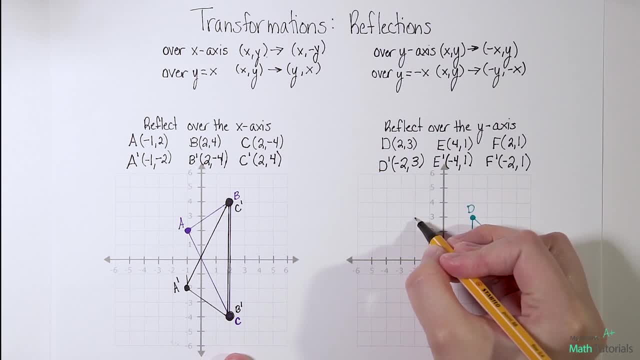 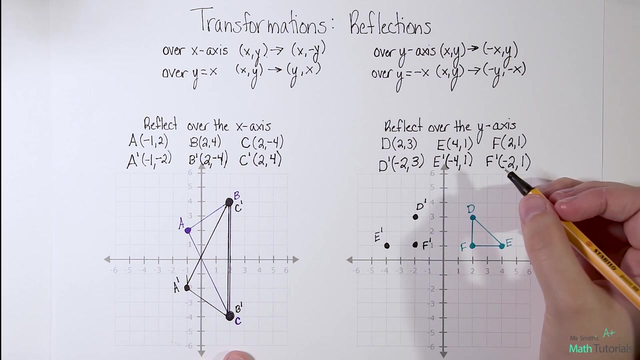 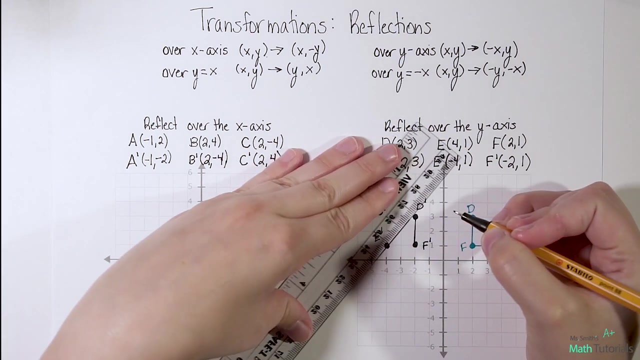 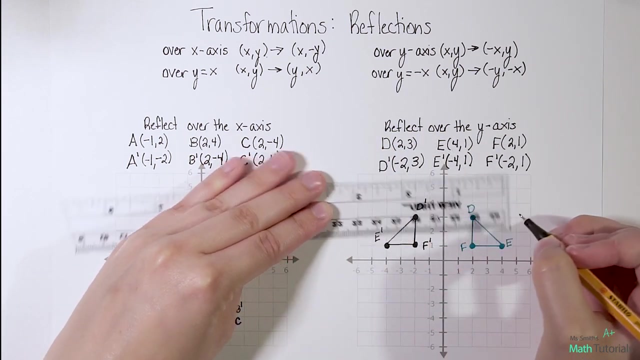 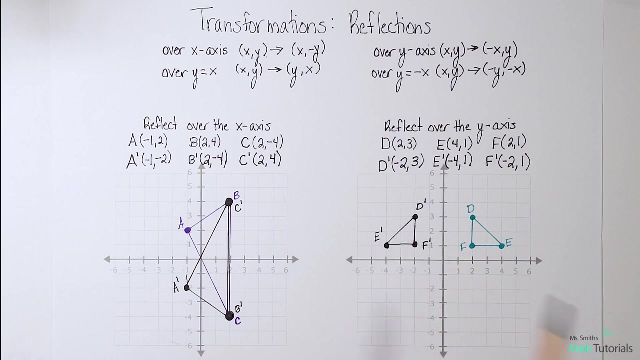 let's see: negative 2, 3- that is our D prime. labeling is so important- e negative: 4: 1. that is our e prime and our F negative: 2, 1 F prime. all right, let's go ahead and connect the dots. okay now. as you can see, it was perfectly reflected over the y axis. it's like the y. 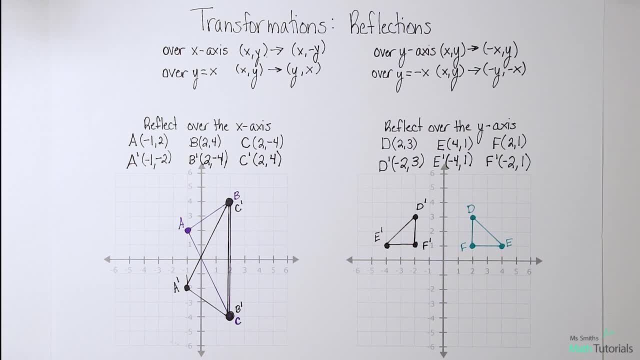 axis is a mirror. now some students like to use the strategy and it is a quicker strategy. they like to take the original picture and just count to the y axis. so now let's go ahead and connect the dots and let's see negative 1 and negative 5 and negative 7. 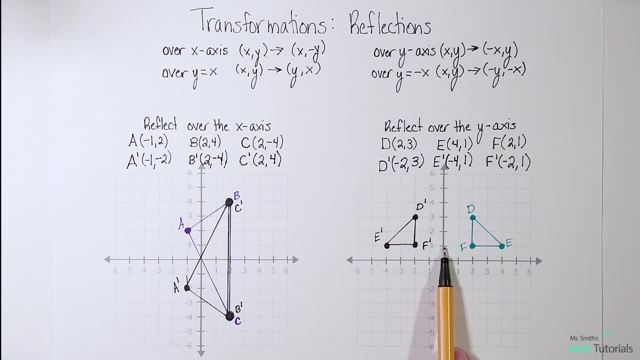 notice, from F to the y-axis I moved over two units, So then they just count two units in the opposite direction: one, two to get to F. You'll notice the same thing with the D and the same thing with the E, even though it's all the way out here. This time we moved in one, two, three, four units. 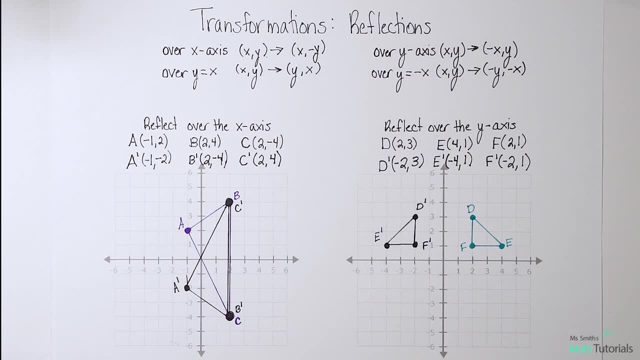 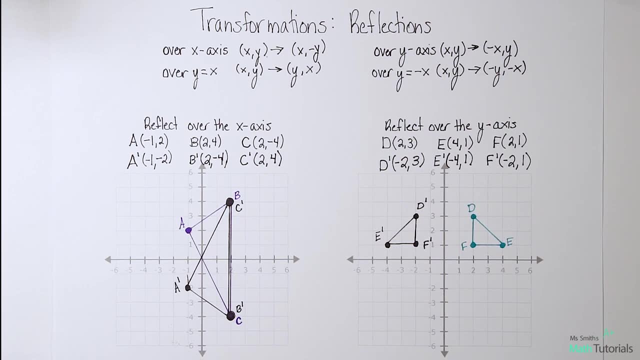 So you would just have to move one, two, three, four units in the other direction. That's totally fine, You can do that. I just like to show the rule behind it so you can fall back on that as well. Let's look at examples now of our other two rules. So for this one, it asks us to reflect this: 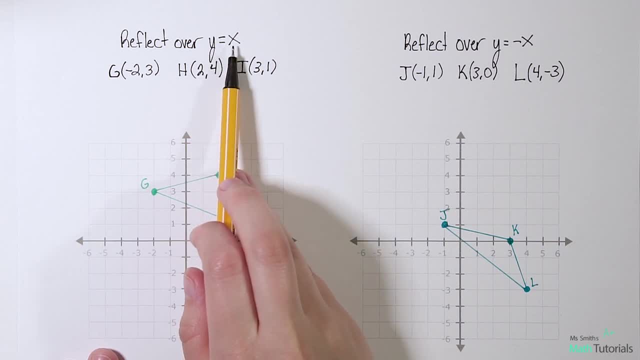 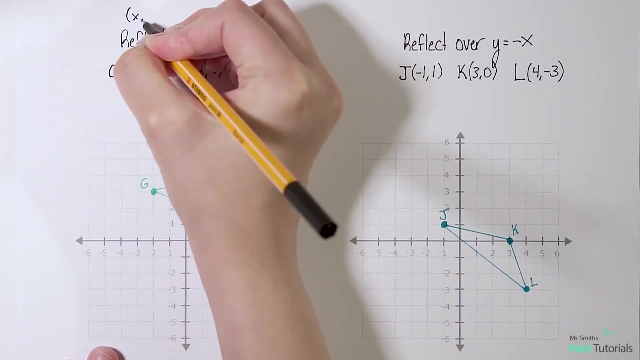 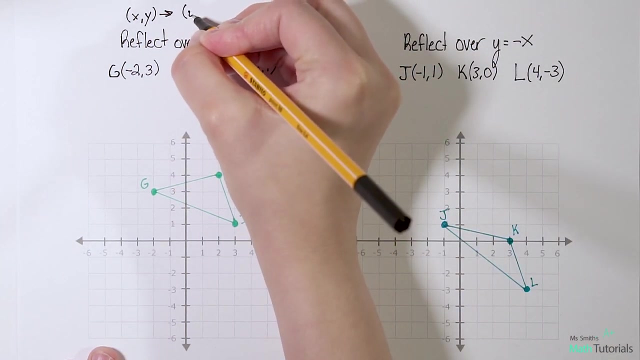 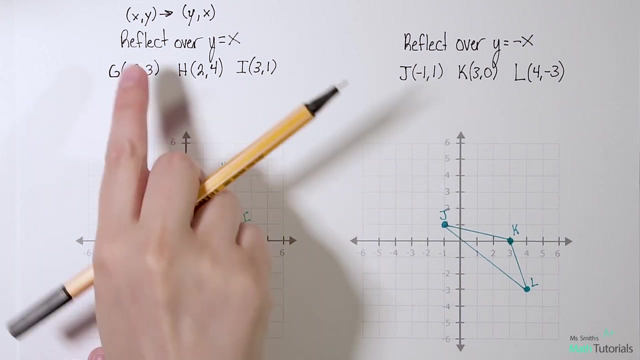 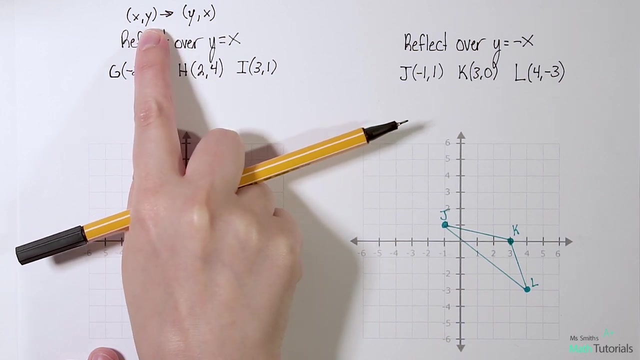 triangle over the line y equals x. Now I'm going to rewrite that rule that was on the other page, just as a quick reminder, so you don't have to scroll back. So xy becomes y comma x. So notice how we just switch The front here. whatever's in the front is going to be in the back, Y is in the back, So whatever's. 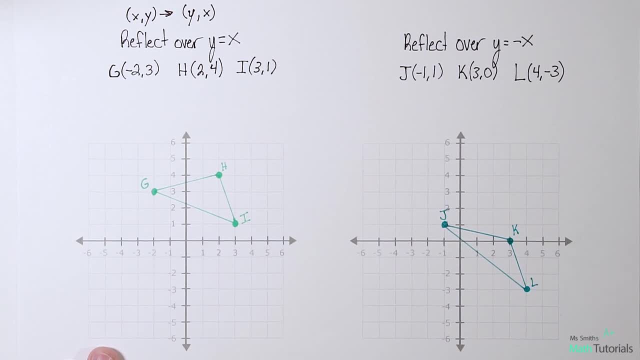 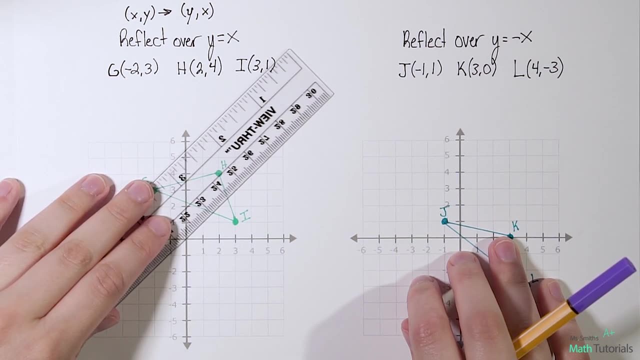 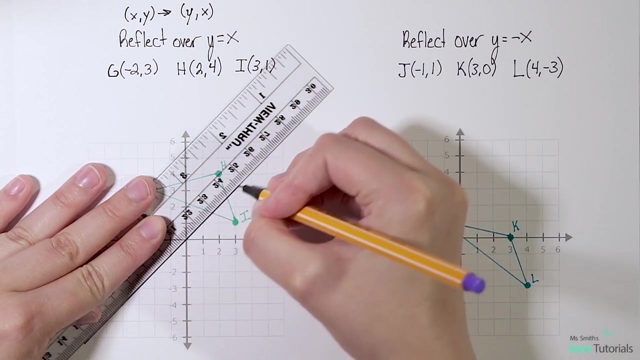 in the back is going to come to the front, So we're just going to switch places, that's all it is. So let's take this one. if I were to create a line diagonally with a positive slope, if I were to 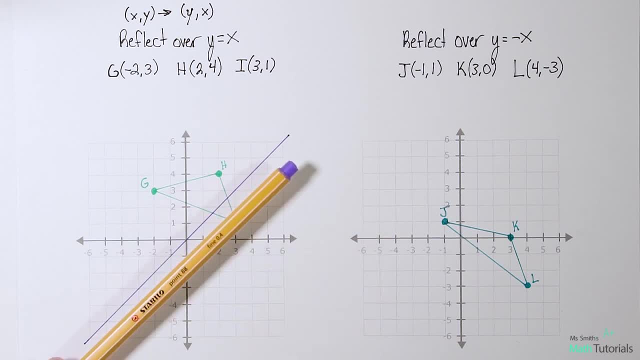 create a line perfectly through, diagonally. through this graph i'm going to reflect this picture over that diagonal line. you can use the counting method. here you would have to count over and down to the line. i prefer to use the rule because sometimes i don't know it can get. 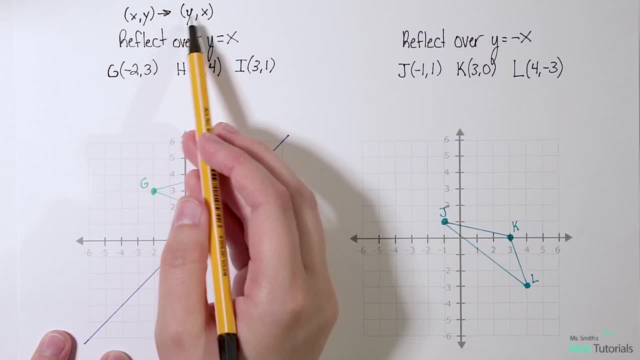 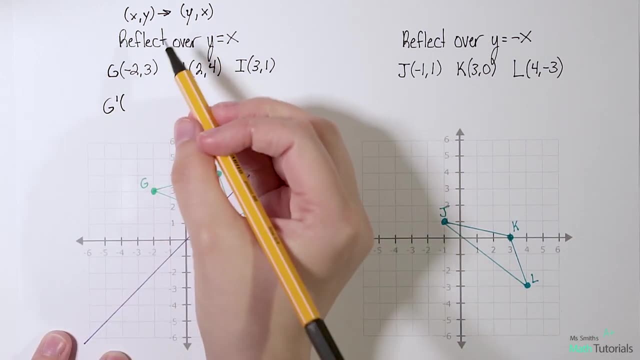 a little complex. so we're just going to follow the rule, this: y, x switching values. so we're going to create a g prime that falls at. we're just going to switch places. the x is going to go to the back, the y is going to go to the front. so three comma negative, two. for h, we're going to create an h. 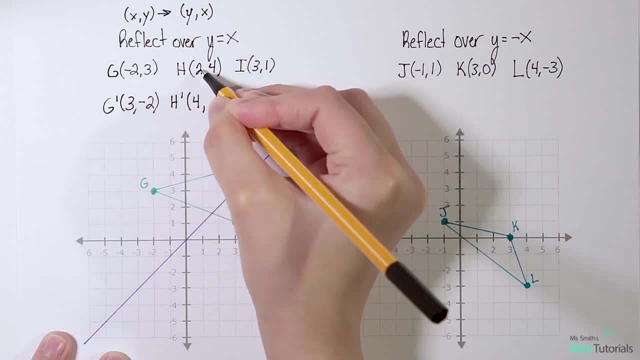 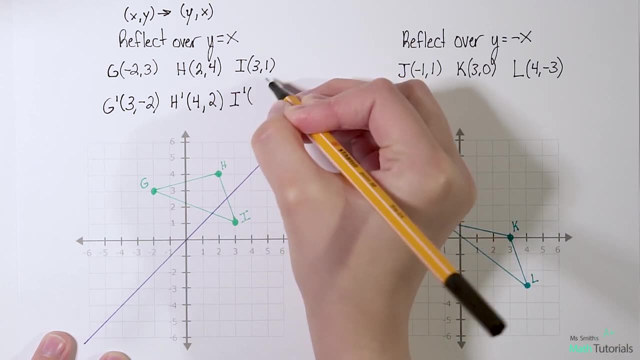 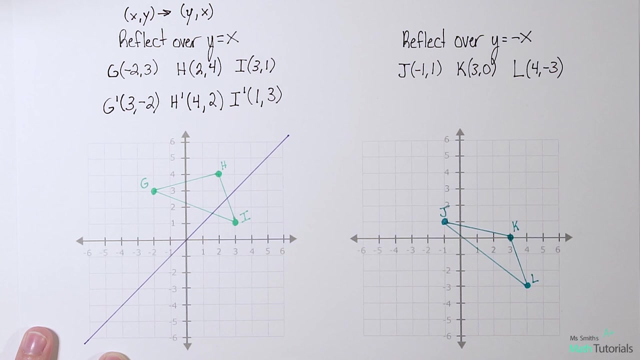 prime. the four is going to come to the front, the two is going to go to the back. and there's our new h for i prime. the one's going to come to the front, the three is going to go to the back. all right, so now i've got my um new image points. let me go ahead and plot them and i 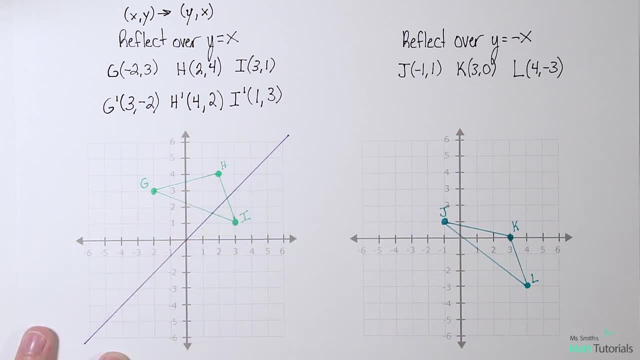 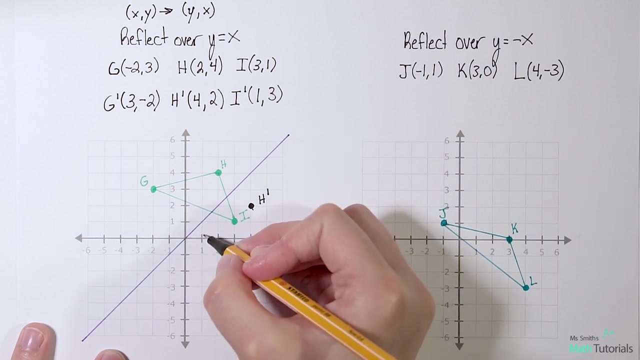 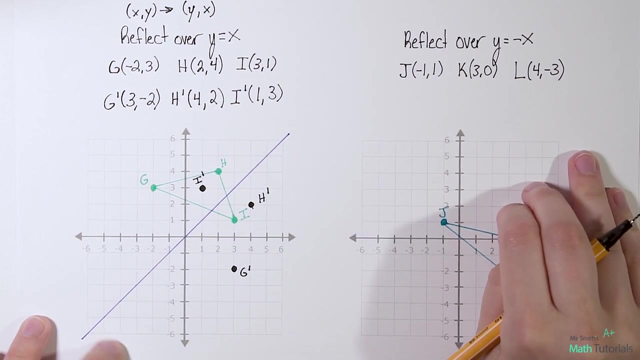 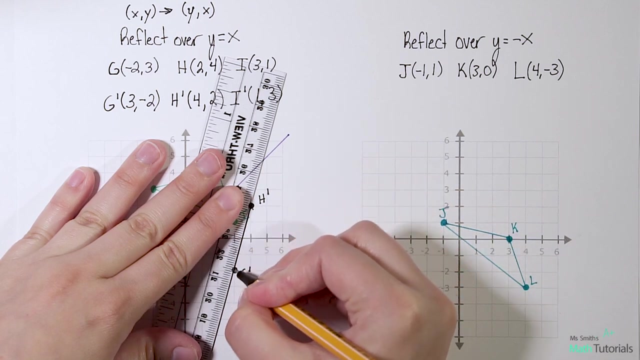 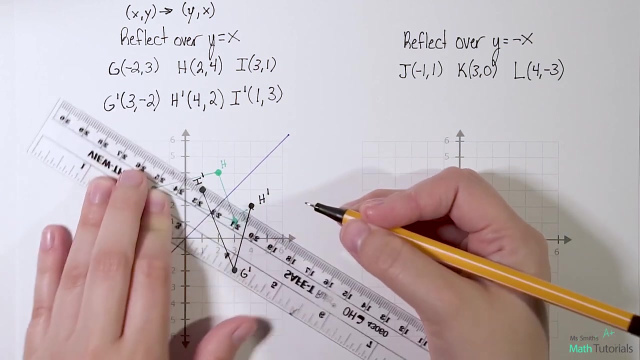 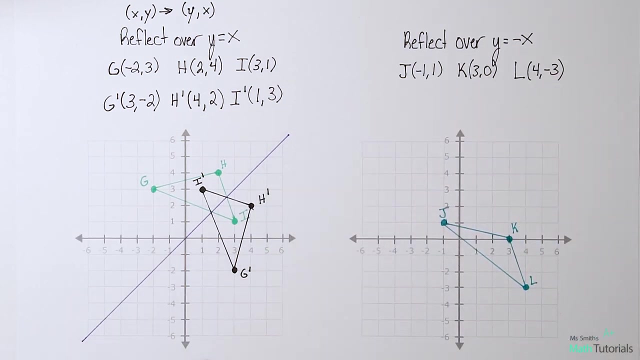 should see that it's a reflection over this diagonal line. so g falls at three negative two. all right, g prime. h falls at four positive two and i falls at four positive two, one, three. let's go ahead and connect the dots, okay, now, hopefully you can see how this is perfectly mirrored over that purple diagonal line that we 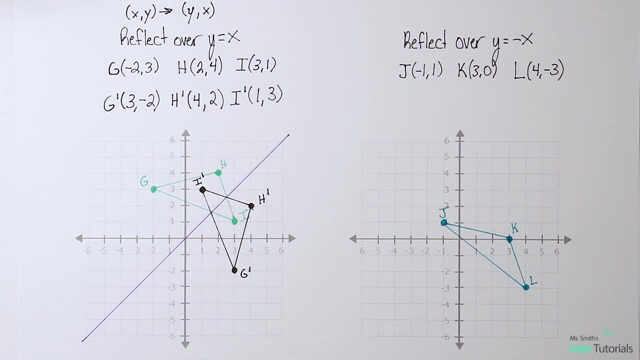 created. that is a reflection over the line y equals x. now let's look at this one over here: reflect over the line y equals negative x, and they gave us a triangle to work with. so this is going to be very similar to this one, only this time we are going to create 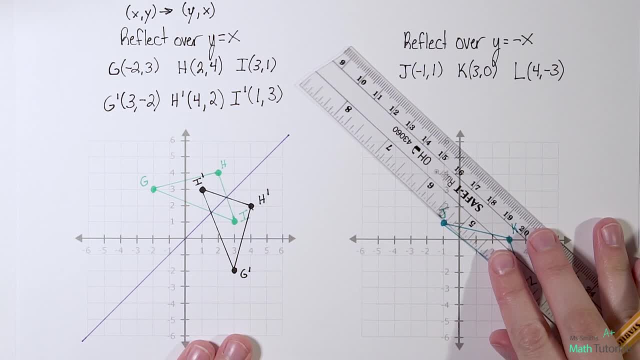 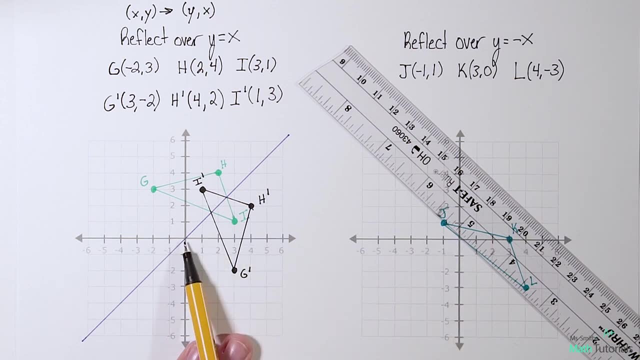 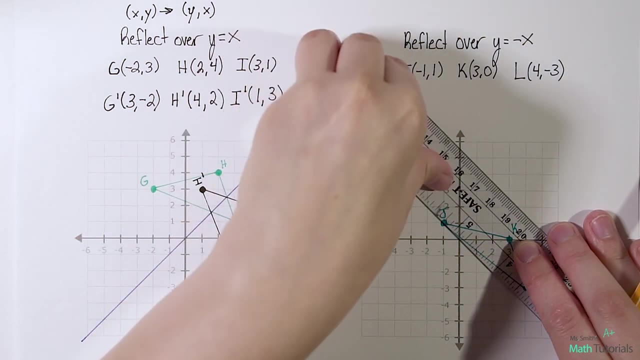 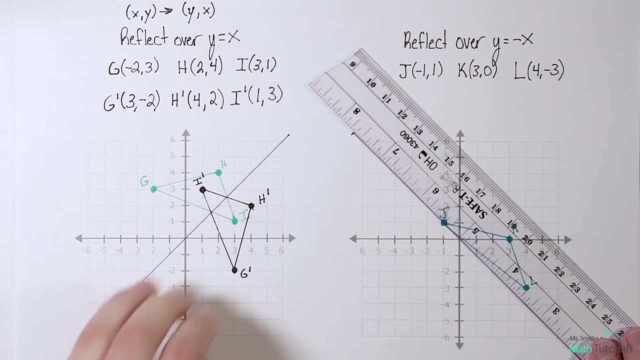 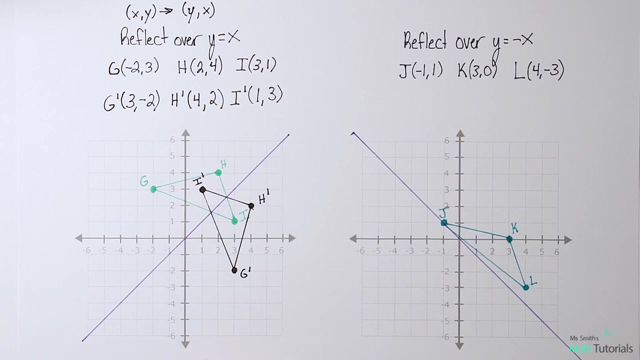 a perfect slope, but it's gonna have a negative slope because this is a negative. so it passes through the origin. it has a y-intercept of zero, just like this one, but the slope is negative. so let me line this up really well. so now, when I create my new shape, it should be reflected over this purple. 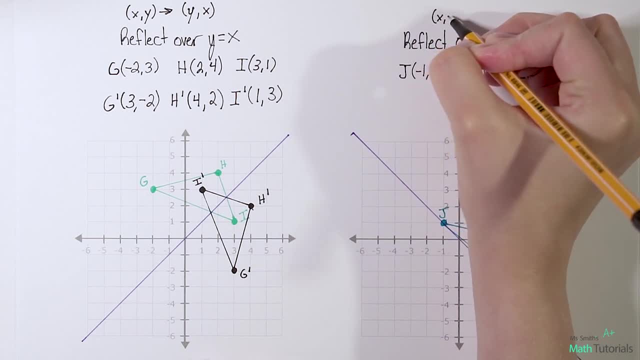 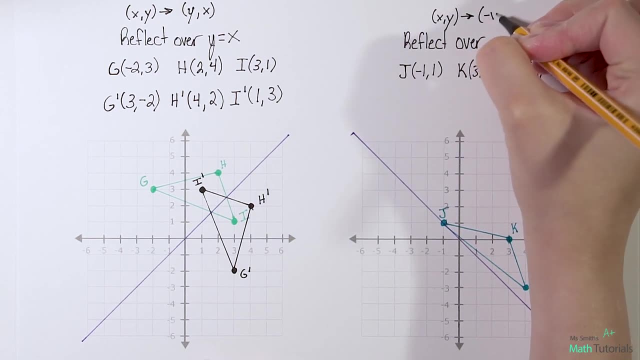 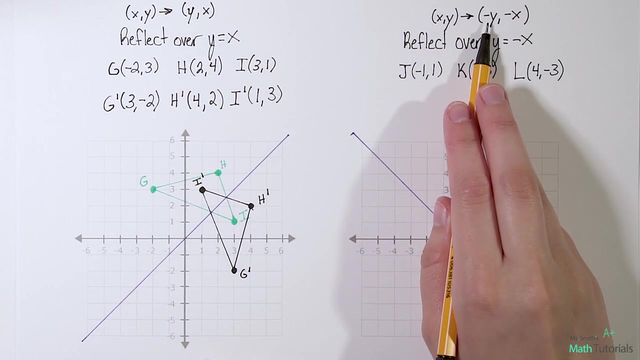 line. so I'm gonna bring over that rule as a reminder from the previous page. X, Y becomes and it is negative Y, comma, negative X. so you'll notice very similar to this one, only this time we switch our signs: Y is gonna come to the front, X is. 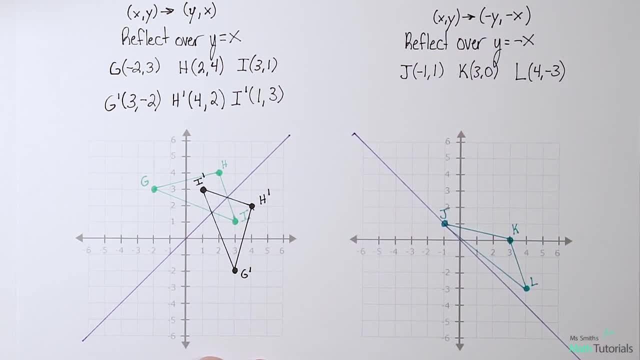 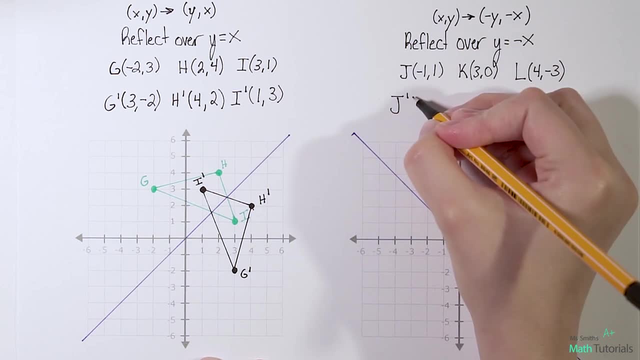 gonna go to the back and we're gonna flip whatever their current signs are, they're gonna become the opposite. so let's see for J: when I create my J prime, my Y is gonna come forward and I'm gonna flip the sign. my X is gonna go to the back and I'm going to 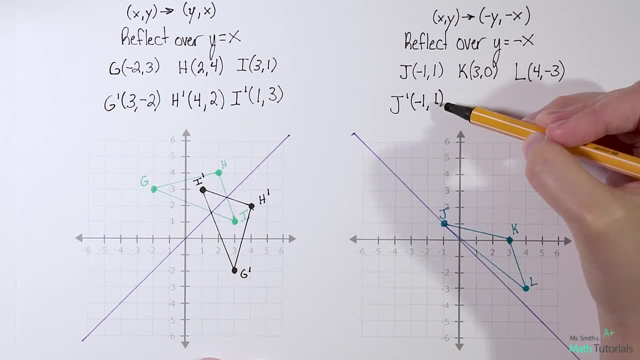 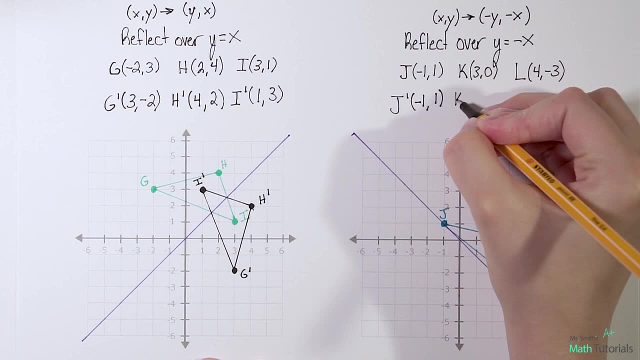 flip the sign. so notice it ended up being the exact same point and that is intentional, that's not a mistake, and you'll see kind of how that works in a second for K prime, my Y is going to come to the front and technically my sign is switching. but we 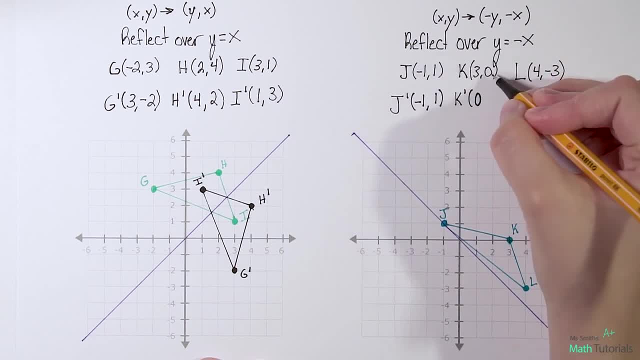 would never have a negative zero, it's just zero. so for that, when we don't have to worry about the sign, three is gonna go to the back and it's gonna become negative for L prime, this negative 3 is gonna come to the front, it's going to. 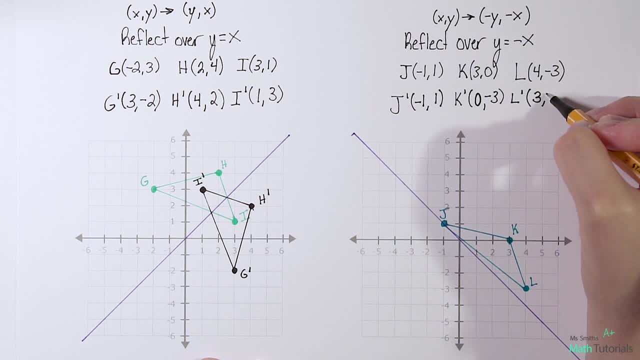 become positive. now flip the sign. the 4 is gonna go to the back and he's going to become negative. Let's now plot our new triangle, our new JKL. So J falls at negative one, positive one, right where the original J did. 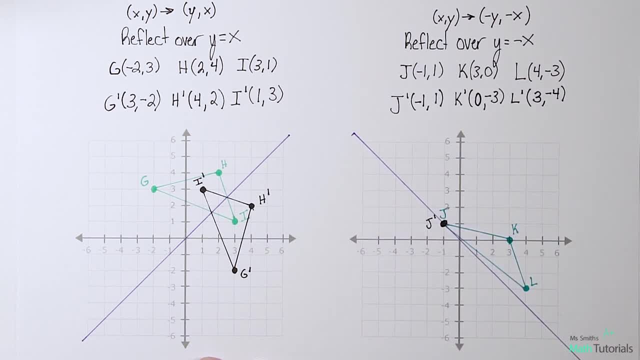 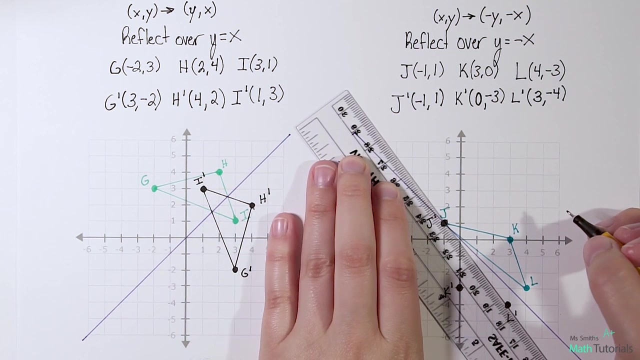 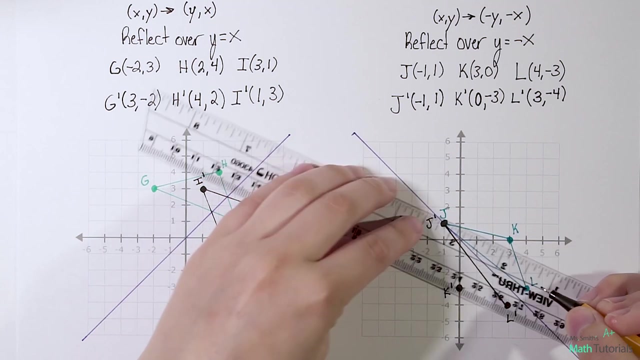 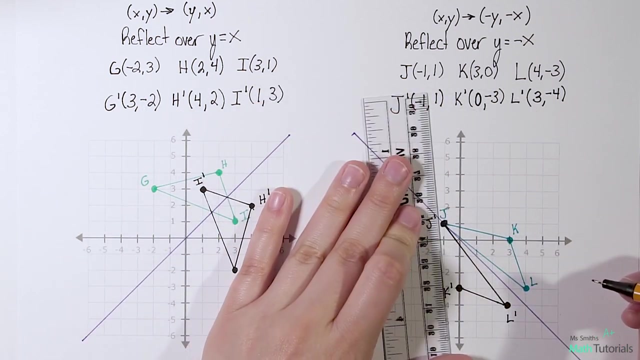 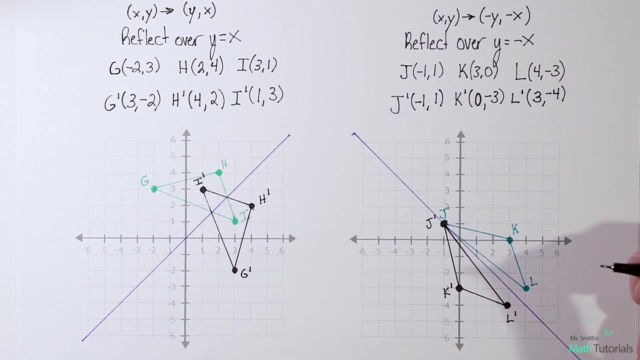 So we'll label that J prime, K falls at zero negative three K prime And L prime falls at three negative four L prime. Let's connect the dots Okay. Now notice how our shape is perfectly reflected over that purple line there. 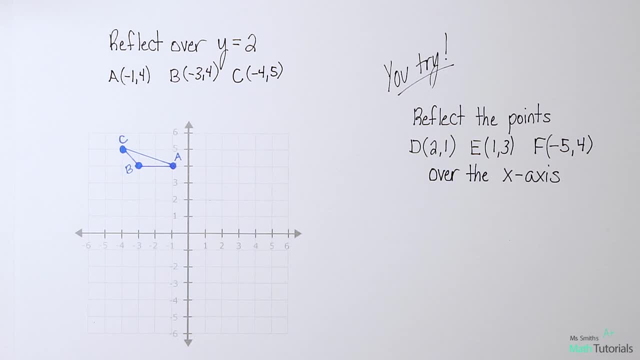 Okay, there's one other type of problem that I wanna show you that you will probably see on your quizzes and tests. Notice this says: reflect over Y equals two. And you may be thinking: well, we didn't have a rule for Y equals two. 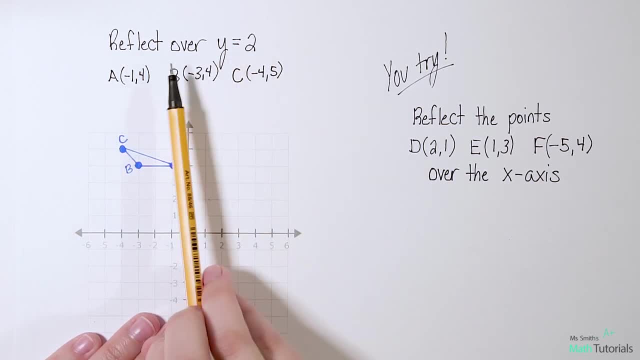 on the first page. We don't, So they will often throw in this line. They are wanting you to mark this line, this equation, on your graph And that's what you're gonna reflect over. So I just happened to pick: Y equals two. 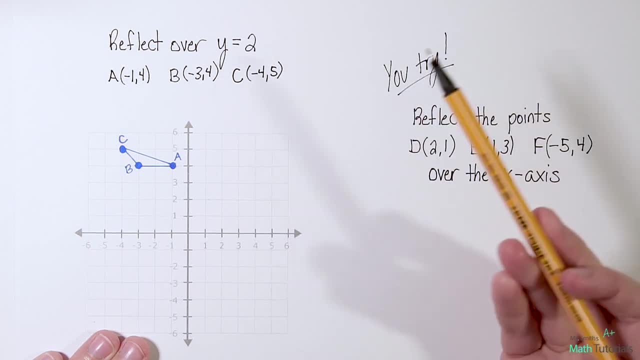 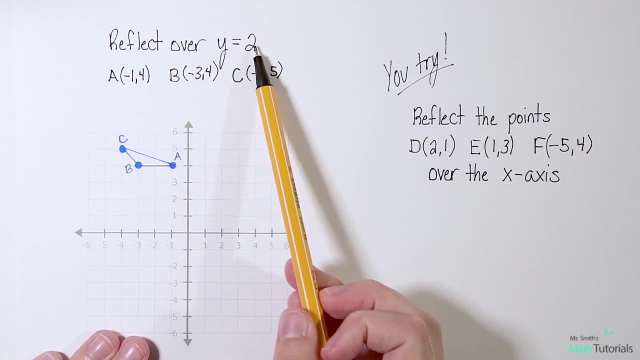 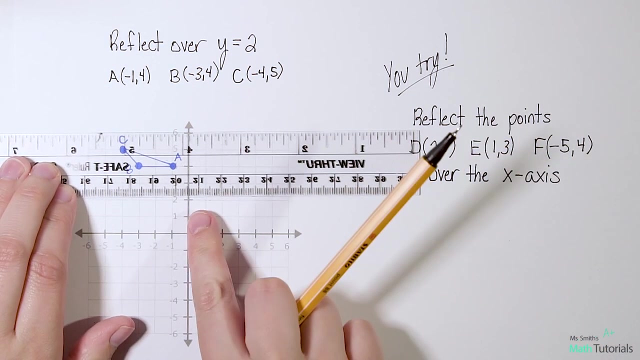 They could give you Y equals five. They could give you X equals one, X equals 10.. Okay, So you wanna remember that Y equals two. that is a horizontal line, So we need to mark that line. It would fall right here where Y is two. 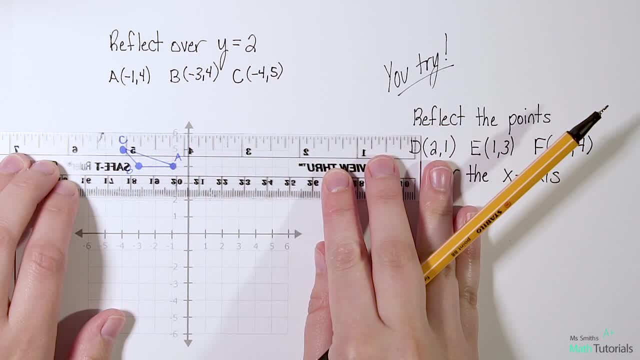 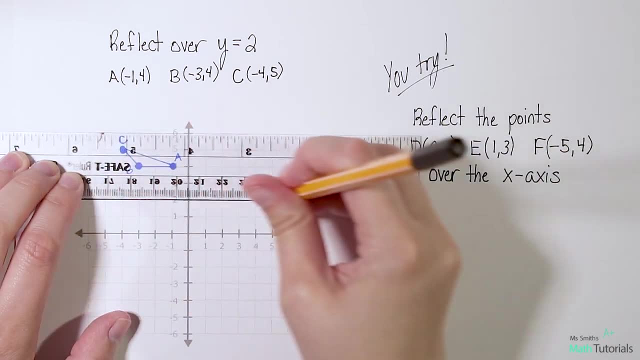 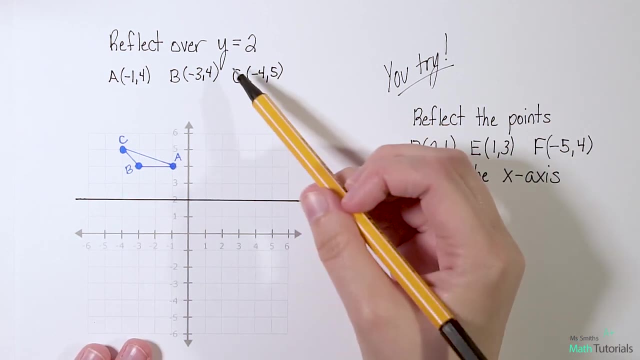 It's a horizontal line straight. It's a vertical line cross. So let's go ahead and mark that. That's gonna be our mirror line for this particular problem, And I wanna make it really dark Now. it's a good thing to note. 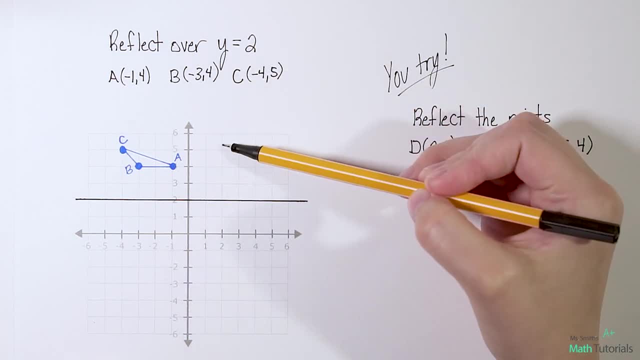 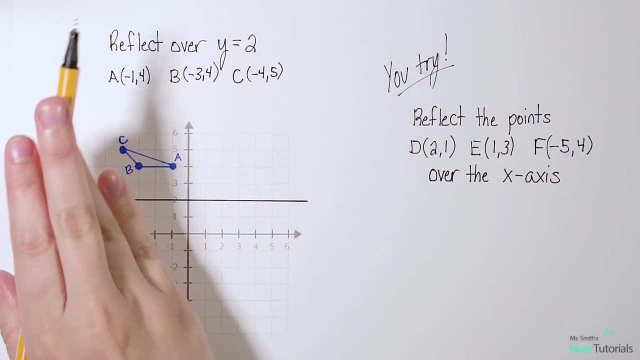 that if they gave you something like X equals two, that's a vertical line. So anytime you have X equals something that's a vertical line, you would just do a vertical line at X equals two, Okay, And it would just be a vertical line. 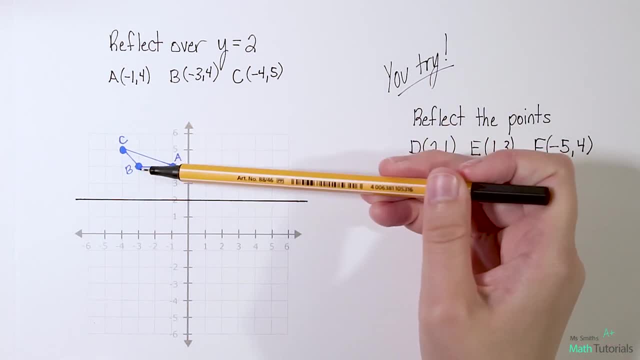 Okay, And it would just be a vertical line. Okay, And it would just be a vertical line. Okay, And it would just be a vertical mirrored image. Okay, And it would just be a vertical mirrored image. But here we're gonna take this image preimage, excuse me. 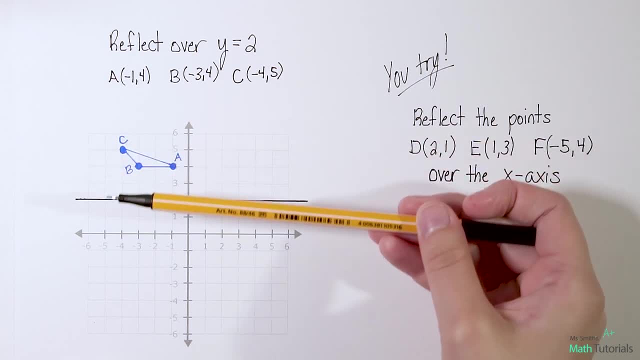 but here we're gonna take this image- preimage, excuse me, for A, B, C- And we are going to reflect it over that line that we just created. There's no set rule for this one. The only way to do this is just to count.